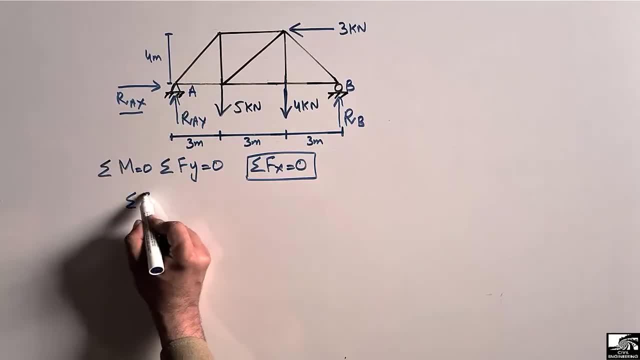 A, X. So summation of horizontal force is equal to zero. So the force is acting in this direction. Let's suppose B take is positive and the force is acting in this direction. Let's assume B take is negative. So all the horizontal forces 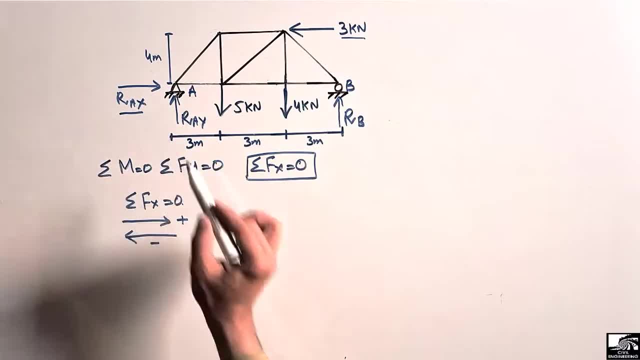 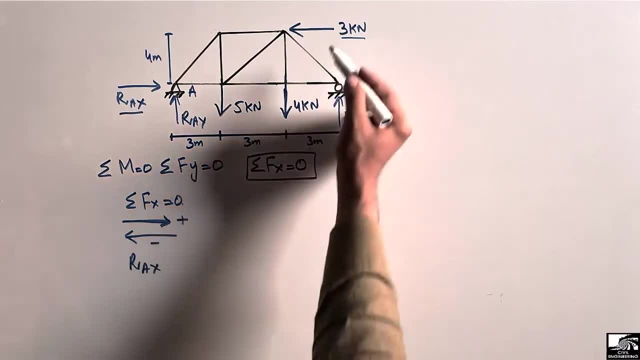 are 3 kN. So now this vertical force of the vertical occurs and this R A X. So this one acting in this direction is this R A X, So it is taken is positive, And force acting in this direction, it is taken as negative, So it is 3 kN, So it will be minus 3.. Summation of 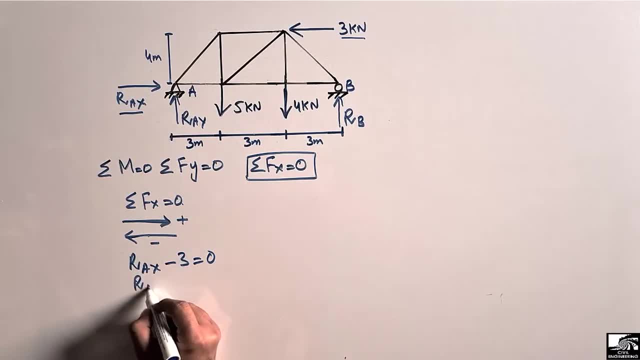 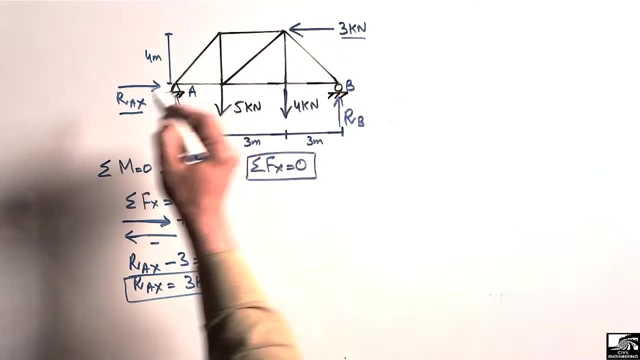 all the horizontal force is equal to zero. So if we shift this into the right side we get R A X equal to 3 kN. So through the whole horizontal load will be taken by this support reaction, Which will be equal to the 3 kN. So we will take the horizontal reaction. 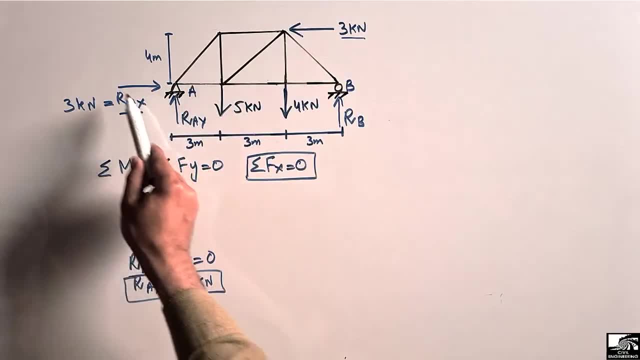 and we will displace all backwards through the Einhorn fielderب or by taking the force. So all the horizontal load is only taken by this support, because it is a hinge support. So it will resist this horizontal load. So it will resist this horizontal load. 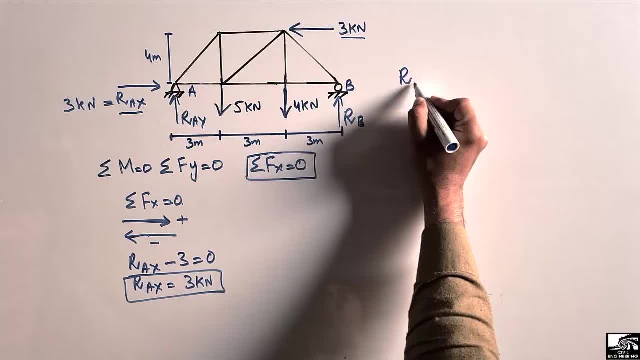 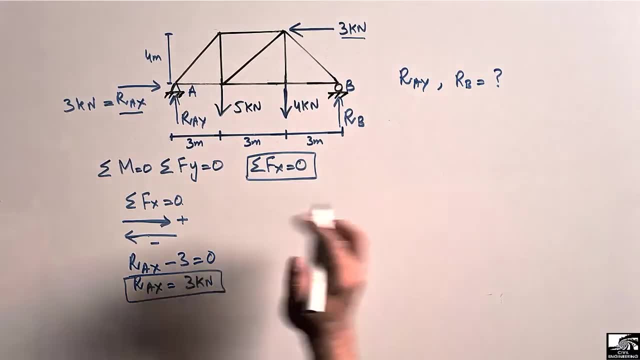 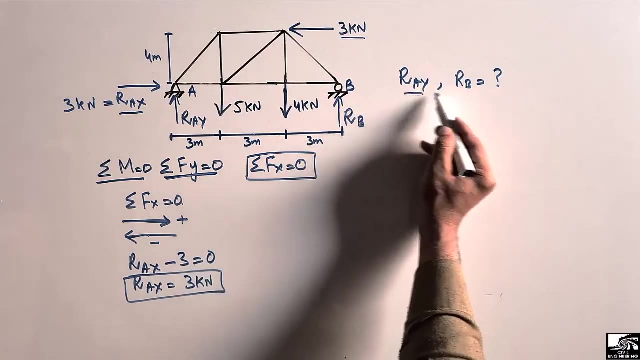 Now to find out the RAY and RB. these two are unknown, So we will use the equilibrium equation of summation of moment, Because this equation can be used when we have only one unknown, But here we have two unknowns. 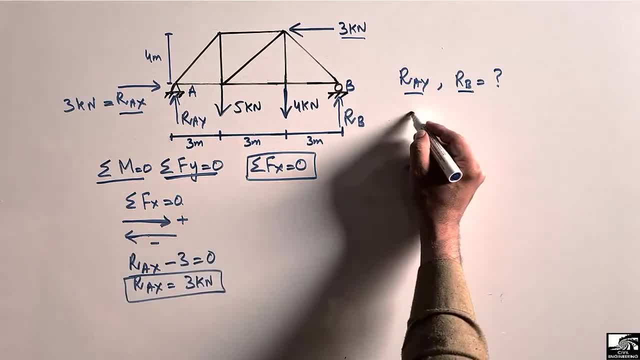 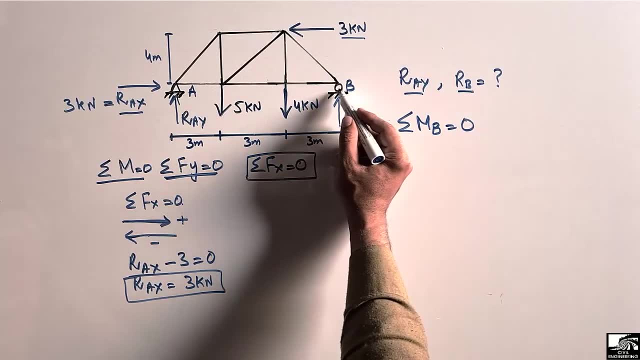 That's why we will use this equation. Now, let's suppose the summation of moment at any point equal to zero. And let's suppose at point B equal to zero summation of all the moment And the clockwise moment is taken as positive, while the interclockwise moment is taken as negative. 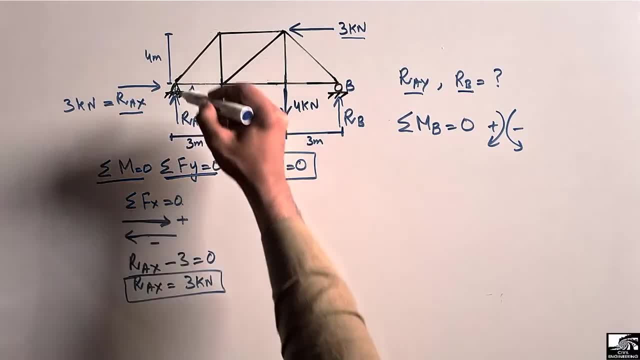 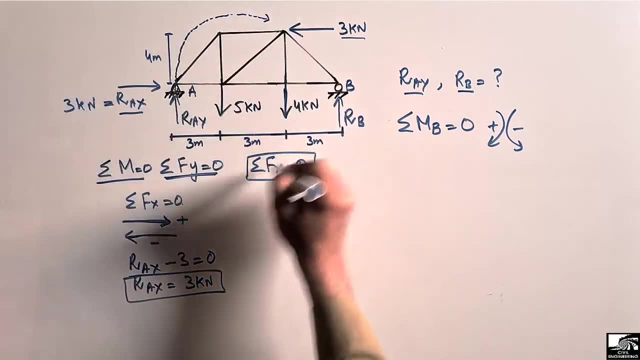 This is just our sign convention. So, starting from this RAY, it is acting in the upper direction, So it will create the moment about point B in the clockwise direction, So it will be taken as positive. So, RAY, 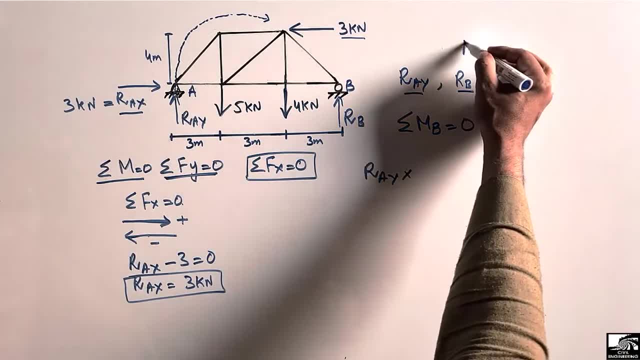 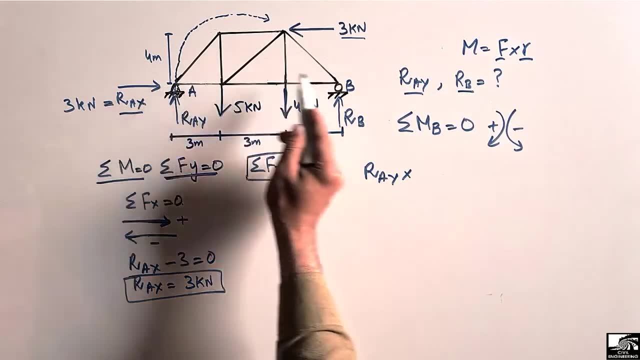 Multiplying it with the moment term, Because moment is equal to the force into moment term. So RAY is the force. Now moment term is the distance from this A point up to the B, Because we want to find out the summation of moment at point B. 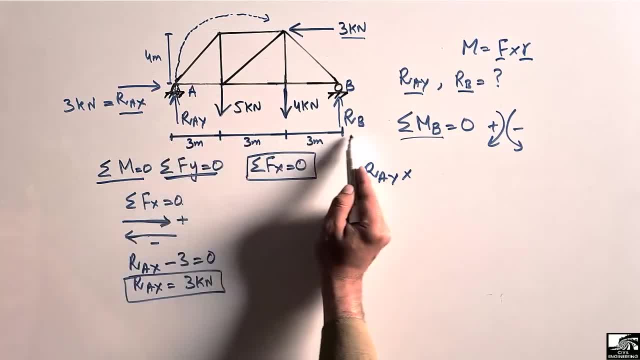 So it is the 3 meter plus 3 meter plus 3 meter, So the total distance is 9 meter. Now this 5 kilonewton will also create the moment about point B, But it will create in the interclockwise direction. 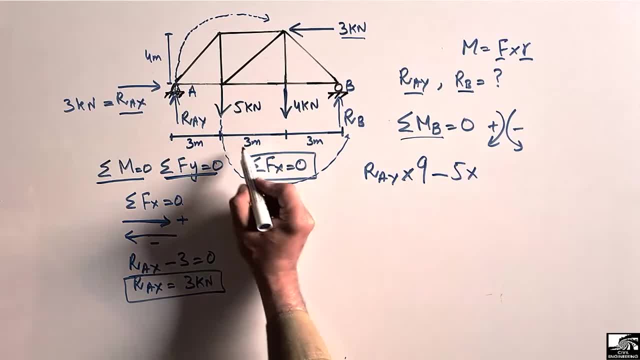 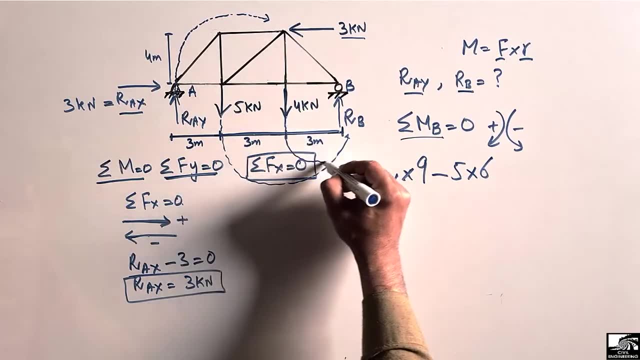 So it will be taken as negative Minus 5.. Into moment term is this distance, Which is 3 plus 3. 6 meter, Now 4, will also create the moment about point B in the interclockwise direction. 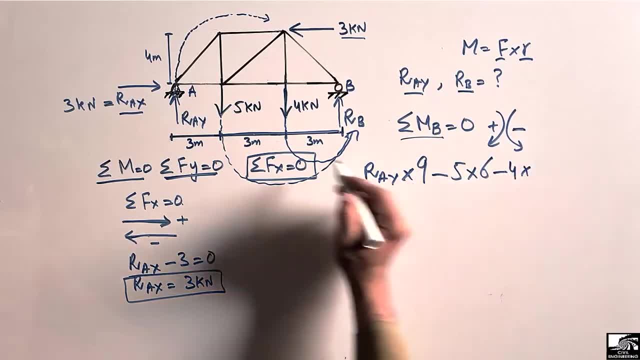 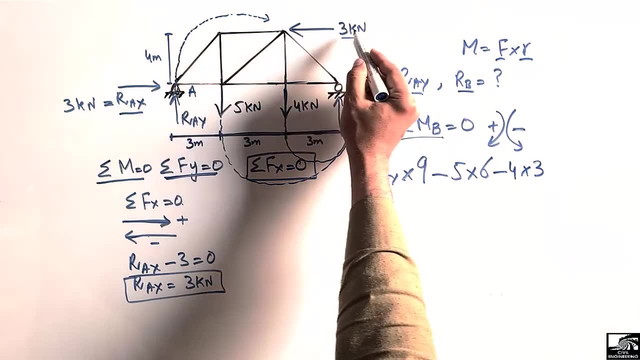 So it will be taken as negative again. So minus 4.. Multiplying it with the moment term, The moment term is the distance from this point up to this point, which is 3 meter. This 3 kilonewton will also create the moment about point B. 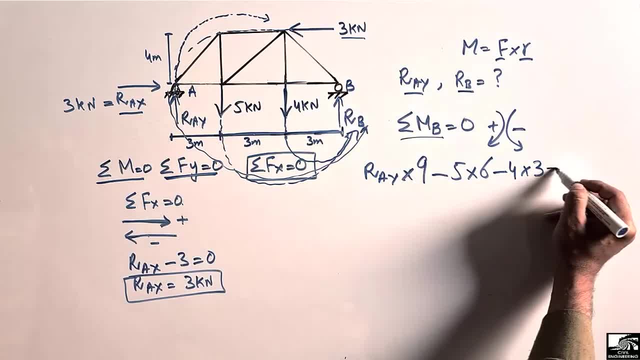 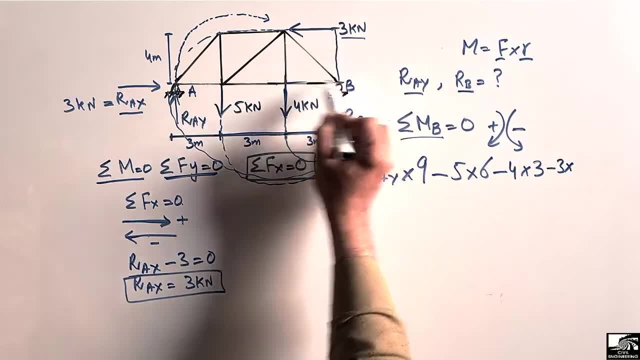 So it will create the moment in the interclockwise direction, So minus 3.. Multiplying it with the moment, The moment term is the distance from this vertical 3 up to point B, which is 4 meter. So summation of all the moment about point B equal to 0.. 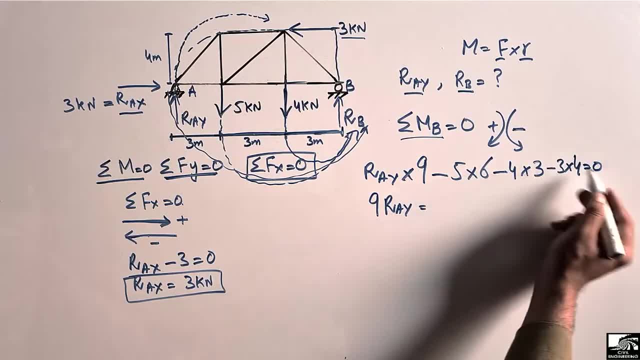 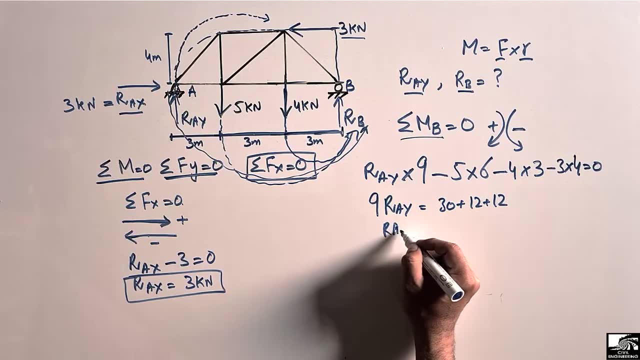 Now 9, Ray. If we shift all these values to the right side, we got 30 plus 12 plus 12.. So by adding these values, Ray, we got 54.. Now, Ray, If we divide this by 9, we got 54.. 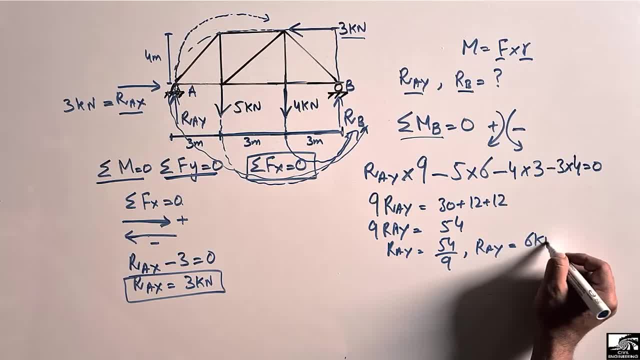 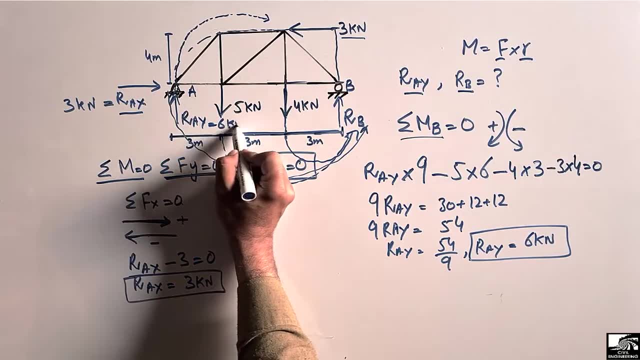 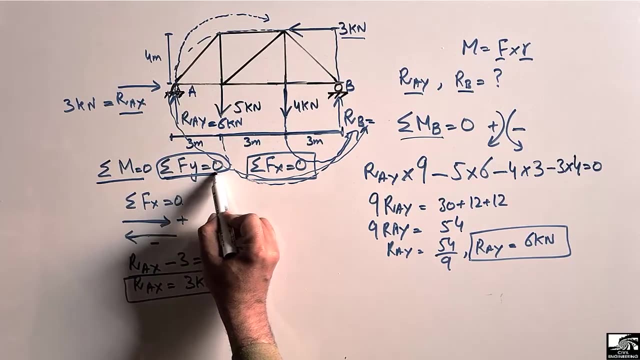 So Ray equals to the 6 kilonewton. So Ray is a support. This support reaction has a magnitude of 6 kilonewton. Now how to find out this Rb? Now we can use distribution in order to find out the Rb. 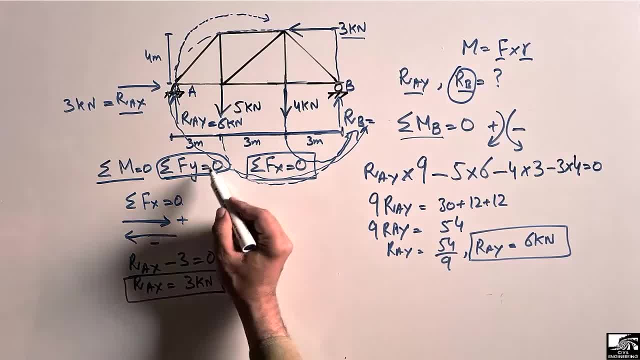 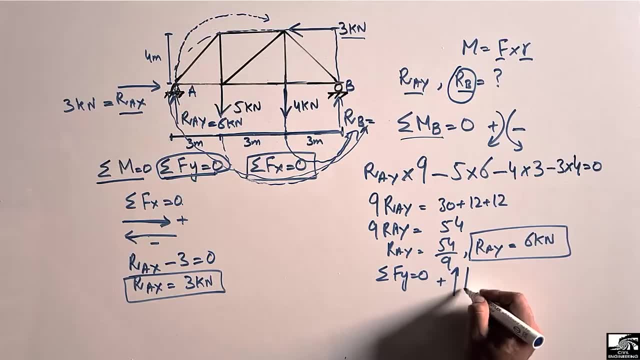 Because now we have only one unknown. So now we can use distribution. So let's suppose summation of all the vertical forces equal to 0. And the upward forces are taken as positive And the downward forces are taken as negative. 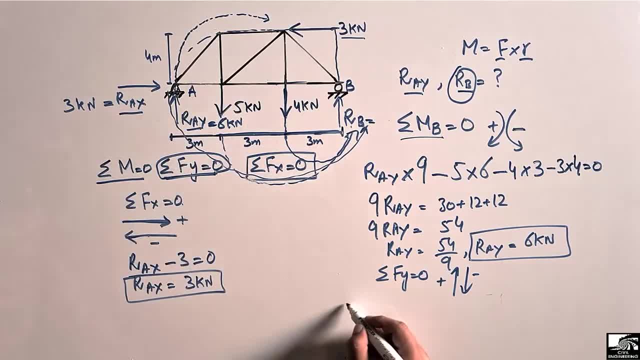 So the upward forces are Ray and Rb. So Ray plus Rb are taken as positive because they are acting in the upward direction And minus this force is acting downward. 5 kilonewton and 4 kilonewton. 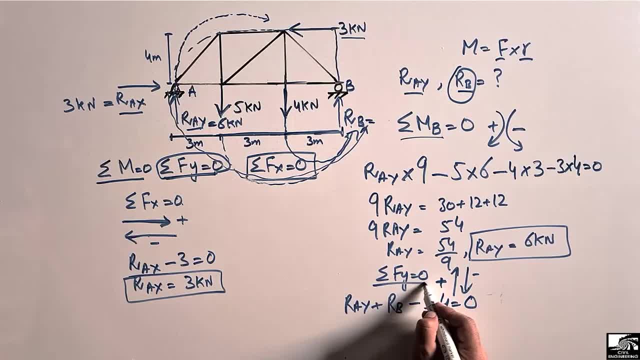 So minus 5 minus 4.. Summation of all the vertical forces equal to 0. So I make all the forces equal to 0. Now Rb will be equal to the. If we shift all these values to the right side, we got 5 plus 4 minus.